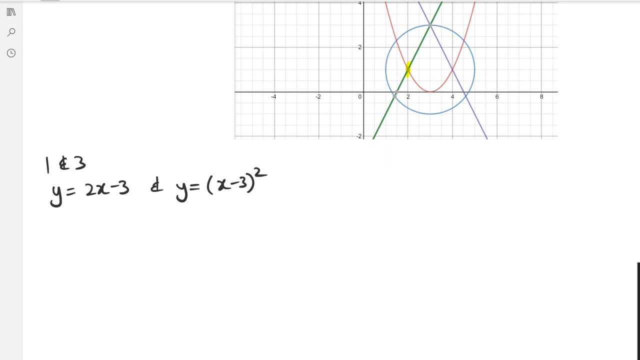 Okay. so with this video, what I'll do is I'll also have the graphics calculator with me so you guys can actually see the graph, So you can actually see how I get the solutions as well. So because both of these y's I can kind of put them equal. they're there, I can put them equal to each other. So I've got 2x minus 3 equals, x minus 3 squared. 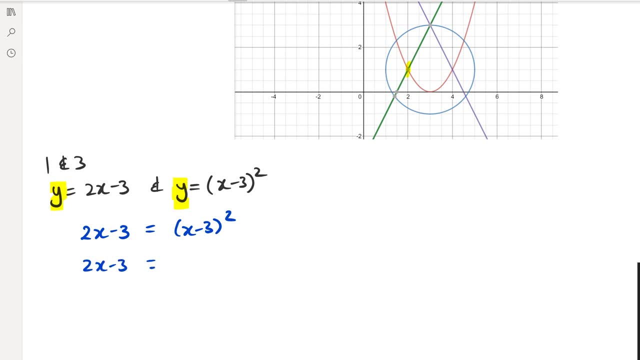 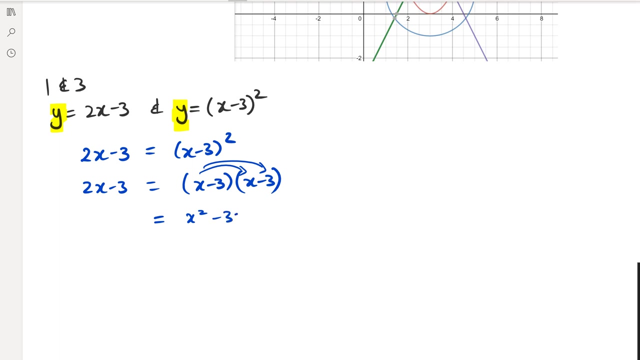 So expand the quadratic. So you've got 2x minus 3 is x minus 3 and x minus 3.. So expand the quadratic. I've got x times x, Which is x squared, x times minus 3 is minus 3x. 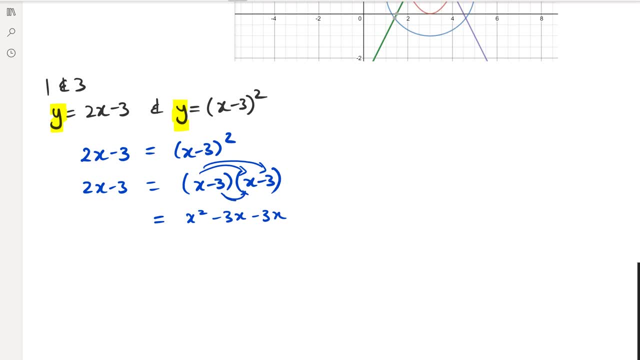 Minus 3 times minus sorry, x is minus 3x, And then negative 3 and negative 3 is positive 9.. So I've got: 2x minus 3 equals this, Which means I need to rearrange everything so that one side is equal to 0.. 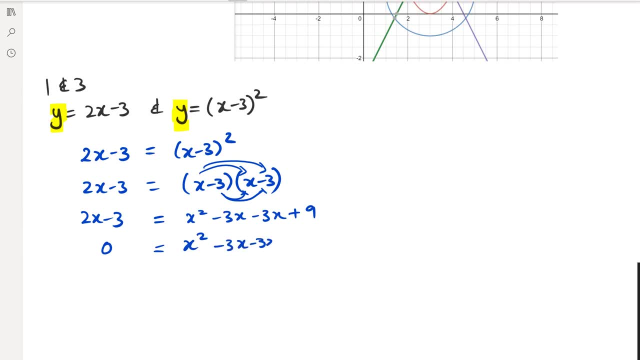 I've got x squared minus 3x minus 3x plus 9.. And then the 2x from the other side, which becomes minus 2x, Negative 3 becomes plus 3.. So, simplifying this, I get: 0 equals x squared minus 8x. 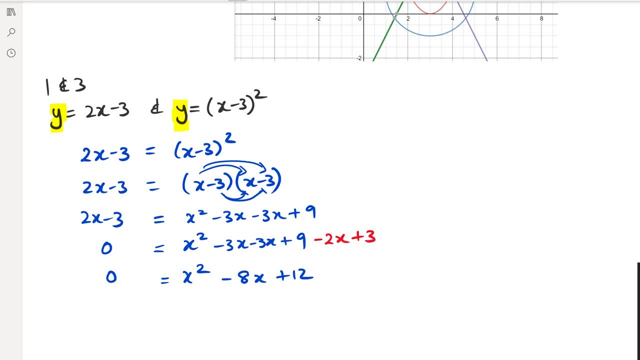 9 plus 3 is 12.. Now, at this point I mean, if you can actually see that, you can factorize it straight away. But if you're not comfortable with it, have your graphics calculator opened up, Go into equation. 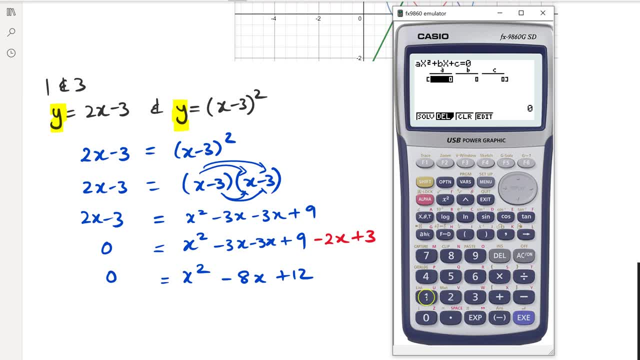 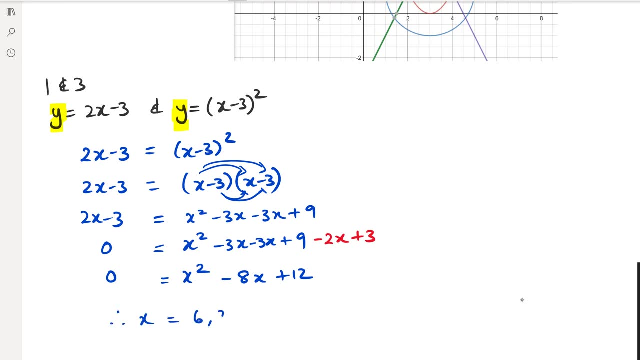 What have we got? Polynomial 2 degrees And our a value is 1. Our b value is minus 8.. And our c value is 12.. So when we solve that, we actually get 6 and 2.. So that means we can say that x is equal to 6 or 2.. 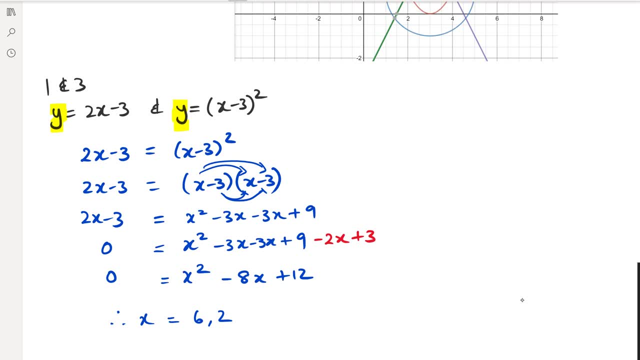 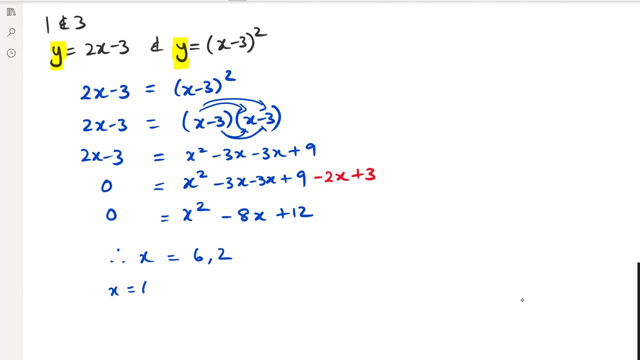 Okay, Now, that's not enough. You've actually got to figure out what the y value is. So what you've got to do is you've got to actually put: when x equals to 6, y is equal to. I'm going to choose the straight line, guys. 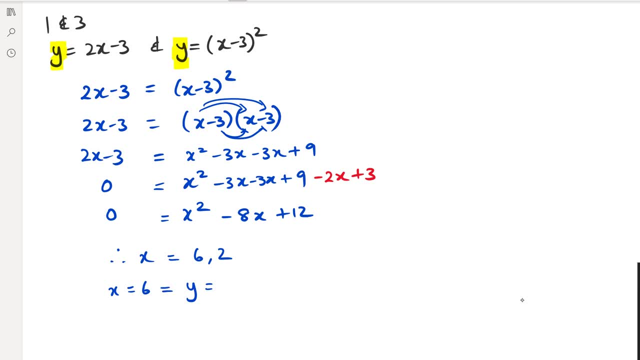 because it's easier to kind, of easier to substitute. So I'm going to say: y equals to 2x minus 3, which means I'm going to get 2 times 6 minus 3, which is 12 minus 3, and it's 9.. 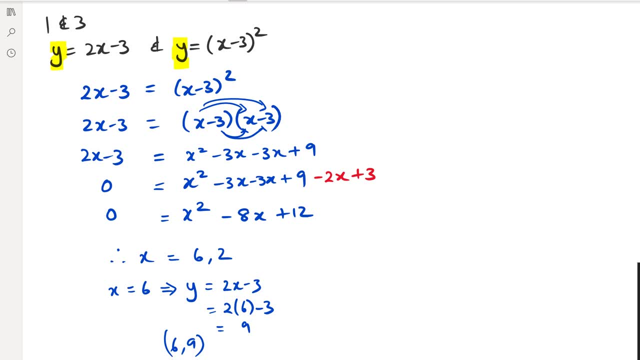 So my first point is 6, 9.. And then, when x equals to 2, I put in: y equals to 2x minus 3. again 2 times 2 minus 3,, which is 4 minus 3,, which is 1.. 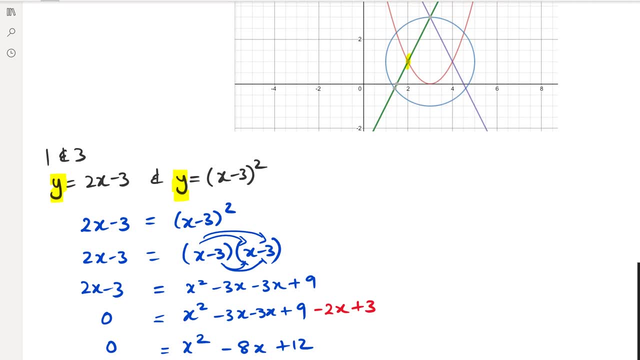 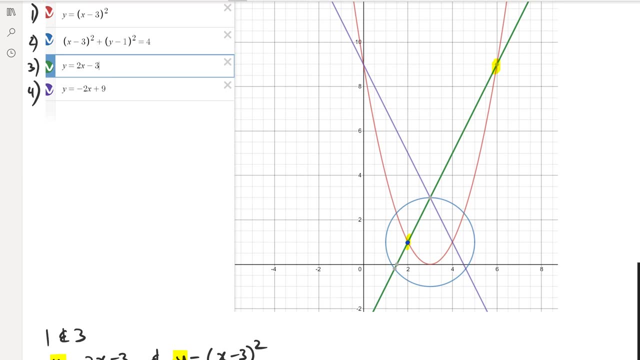 So I've got the point 2, 1.. So if you guys go back and have a look at the two yellow dots there, you can kind of see that it's actually at that point right there. I'll show you guys in Desmos itself so you can have a look. 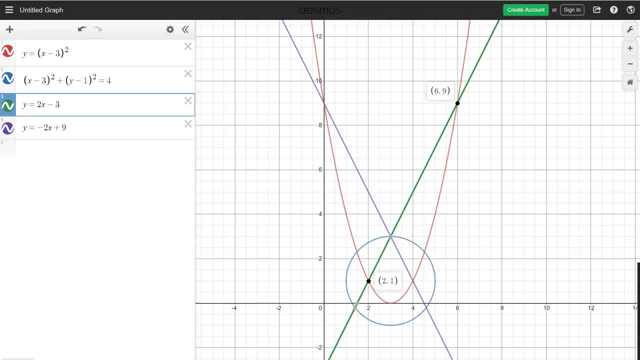 So that's that first point there, which is 2, 1.. And that's that second point there, which is 6, 9.. Okay, So you guys should be able to do that, Like that's going to be nice standard parabola and straight line matching. 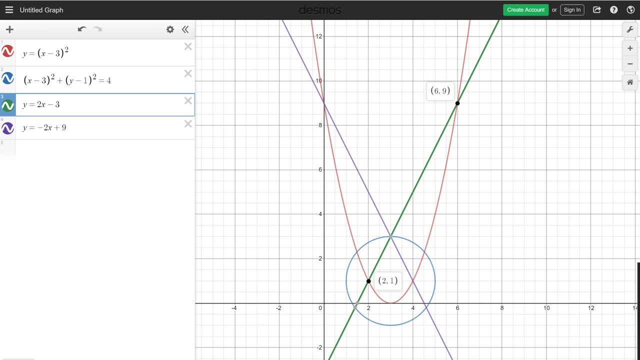 Now, if I was to do it with the purple line and the red line, it's pretty much going to be the same thing, All right, So I'm going to get you guys to do that at a later time, But the one that I want to have a look at next is the green line. 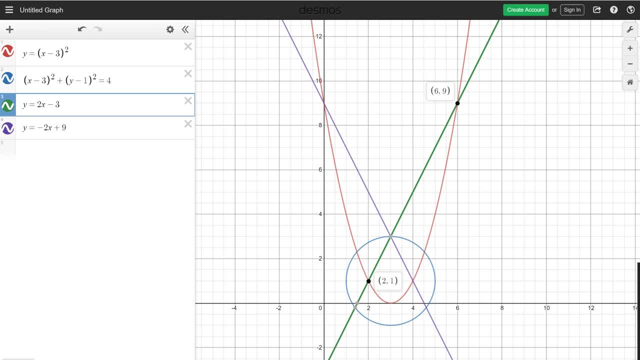 and the blue circle, All right. So basically I'm looking at, let me just say, green and purple, So I'm going to take out this. So I'm looking at the circle and I'm looking at the straight line and I want to figure out where they actually meet. 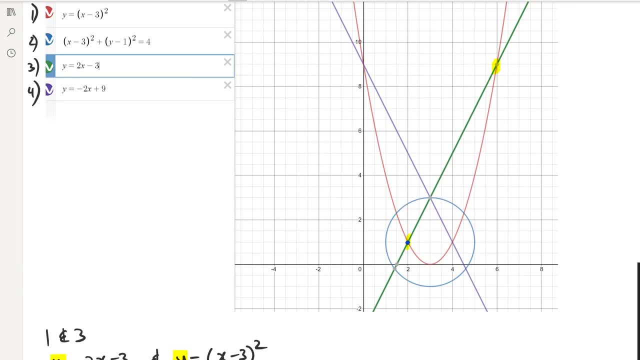 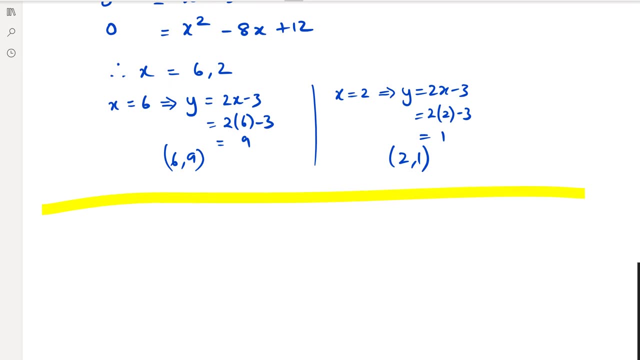 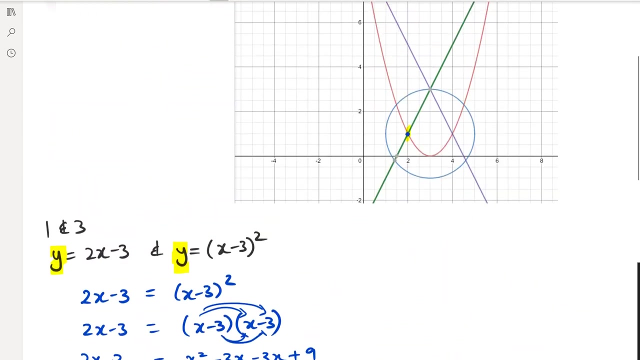 All right, So that's equation number 2 and 3 I'm going to be looking at. So let's go down. So equation 2 and 3.. What are my two equations there? Give me a second man, Okay. 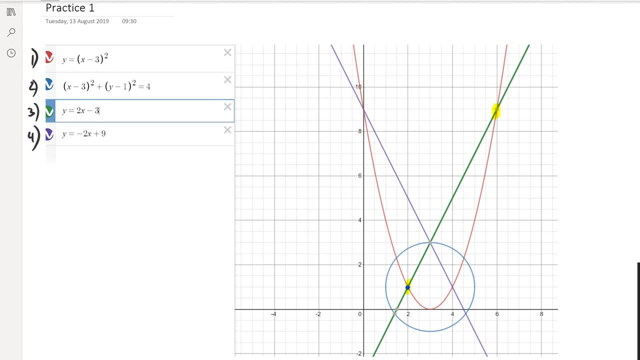 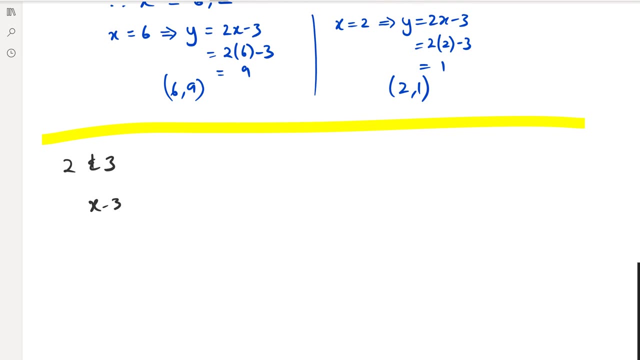 So number 2, what we have is we've got the circle and then we've got the straight line again. So we're going to kind of have a look at that. So Okay, So Okay. So my circle's equation is: x minus 3 squared plus y minus 1 squared equals 4.. 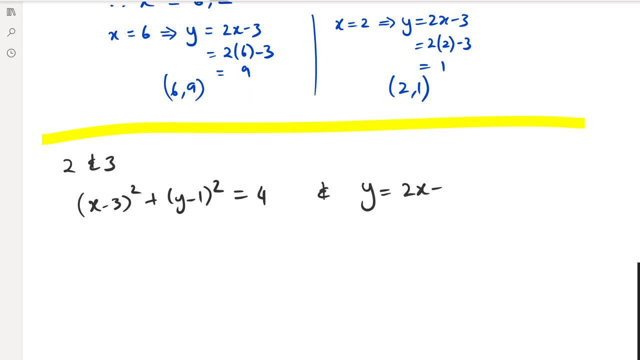 And then the straight line equation is: y equals to 2x minus 3,. right Now this part. watch what happens, guys. There's nothing really changes than what you did from the previous one. It's just this one little extra step that you've got to do. 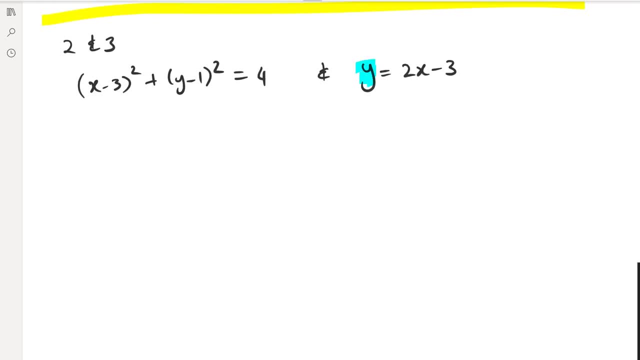 So the step is this: Right now you've got y is equal to 2x minus 3.. That means you can actually replace the y here. Notice how I've highlighted all of them in the blue color, which means everything in the blue color is the same thing. 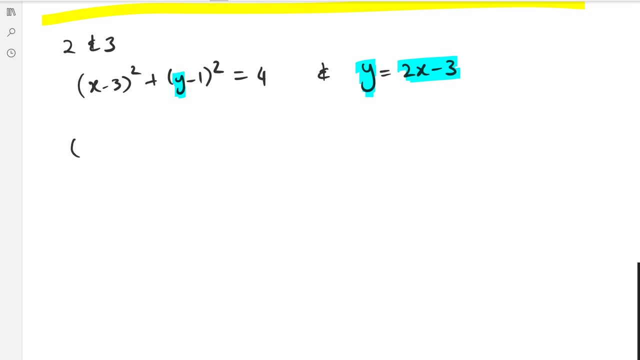 So that means I can rewrite this equation now as x minus 3 squared plus. instead of writing y, I actually write 2x minus 3 minus 1 squared equals 4.. So notice what I've done here. I've actually replaced y. 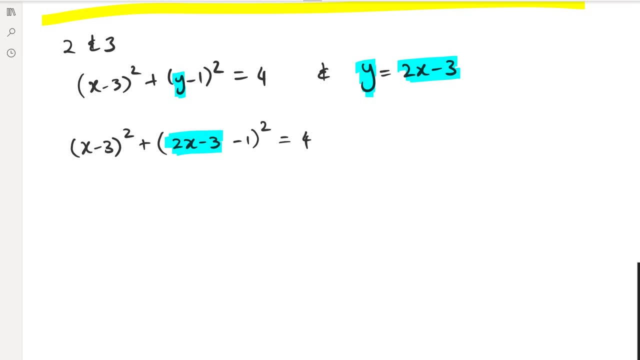 That entire y with 2x minus 3.. Okay, So that's all. Then it's just expanding the quadratic, simplifying it and solving it. So what I've got here. but remember, with this second bracket here you've got this one extra step to do now. 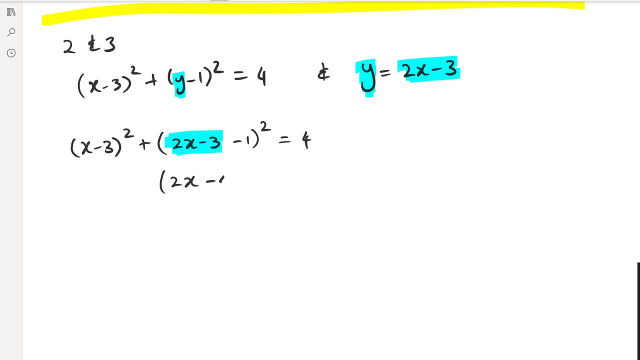 So you've got to go 2x minus 3, and minus 1 will actually become minus 4.. Okay, And then. so that's it. So I've got this 2x minus 4 squared, and then here I've got x minus 3 squared, plus equals to 4.. 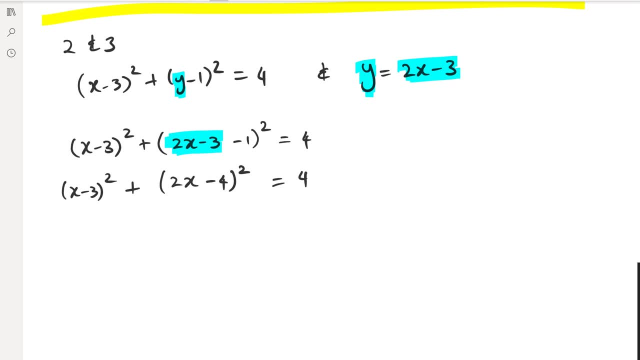 Okay. So all I've done is I've actually got rid of that y and I've replaced it with an x. So at this point I've got a bunch of quadratics again and I've got to expand them. So I've got x minus 3 times x minus 3 plus 2x minus 4 times 2x minus 4.. 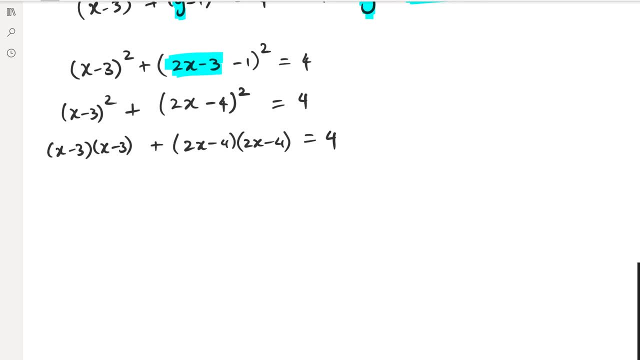 All of that equals to 4.. Okay, So then I do the whole FOIL method again, So I've got x times x, which is x squared, x times minus 3, which is minus 3x, negative 3 and x is negative, 3x negative 3 and negative 3 is plus 9,. 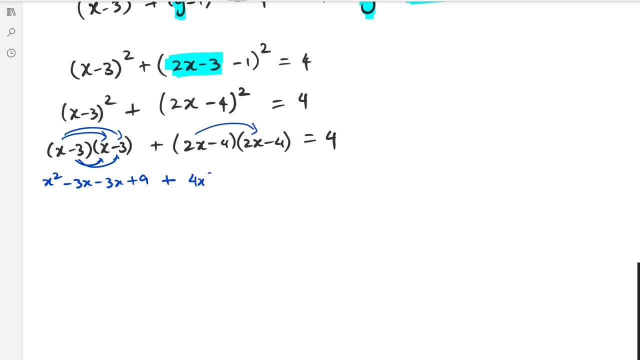 plus. then I've got 2x times 2x, which is 4x squared, 2x times minus 4, which is minus 8x, minus 8x again, and then plus 64. And all of that equals to 4.. 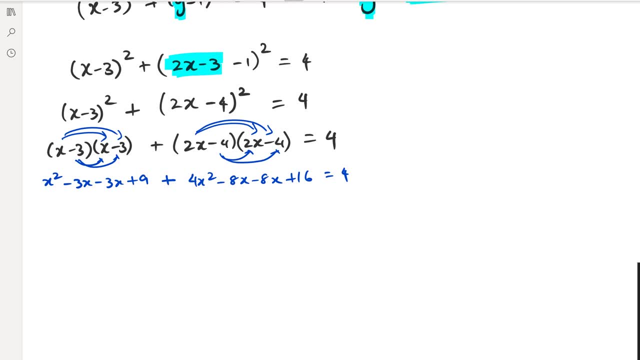 So at this point I want to collect my like terms. So when I say like terms, I'll look at all my x squareds. Okay, There's no more x squareds, So that means that's going to be 5x squared. 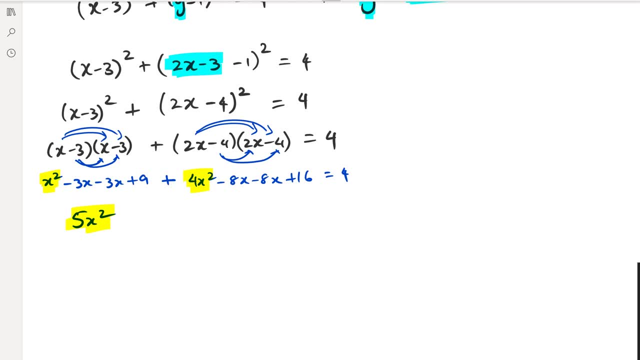 Highlight that yellow. Next, I need to look at all my x's. So I've got negative 3x, negative 3x, negative 8x, negative 8x, And when I combine that I've got negative 6x. 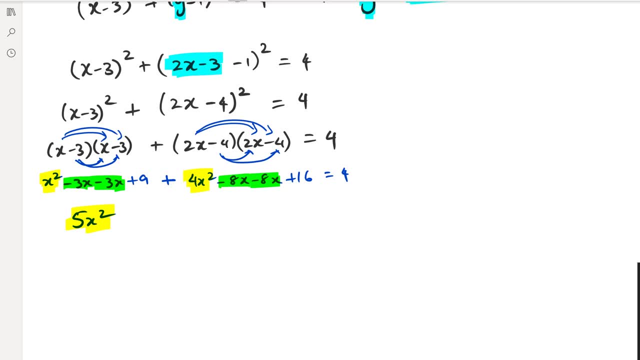 So I've got negative 6x. So I've got negative 6x. Well, we've got 16, 11,, 11,, 22, minus 22x. So that's all the green part that's highlighted. 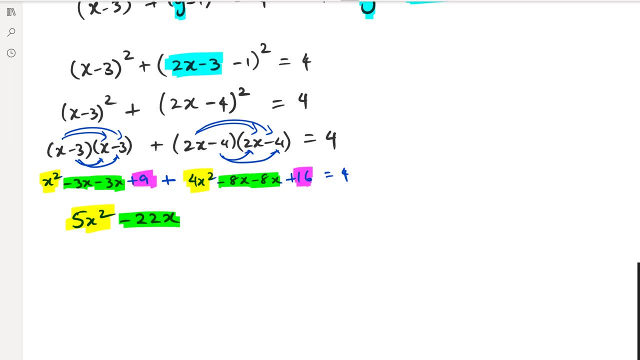 And then finally the numbers by themselves. In this case, I've got 9, positive 9, and positive 16,, which is plus 25.. And all of that is equal to 4.. So I rearrange this so that one side equals to 0. 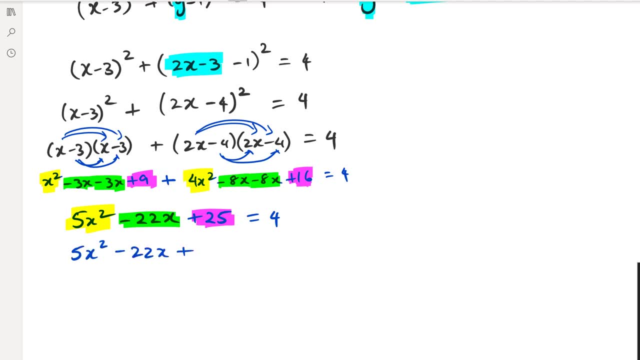 I've got 5x squared. I've got 5x squared minus 22x plus 25.. And then when I bring the 4 onto this side, it becomes minus 4, which equals to 0.. Simplifying it, I've got 5x squared minus 22x plus 21, equals to 0.. 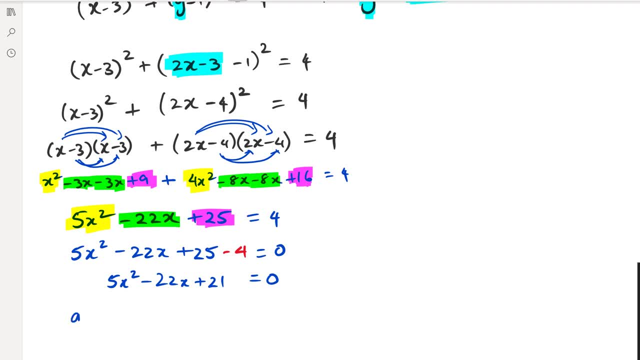 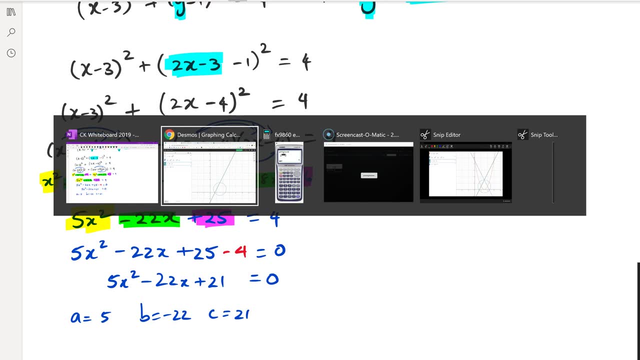 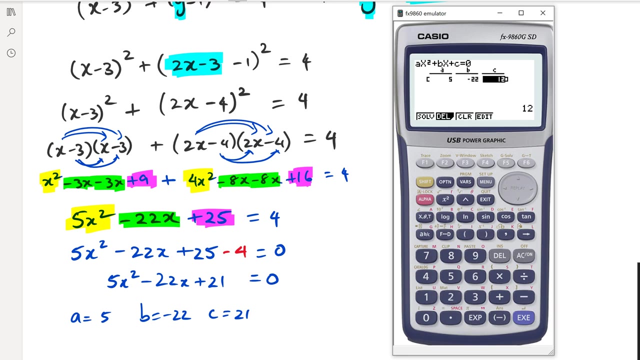 At this point I write down my a, b, c values. So I've got: a equals to 5,, b equals minus 22,. c equals to 21.. So I've got 5, negative 22, and 21.. 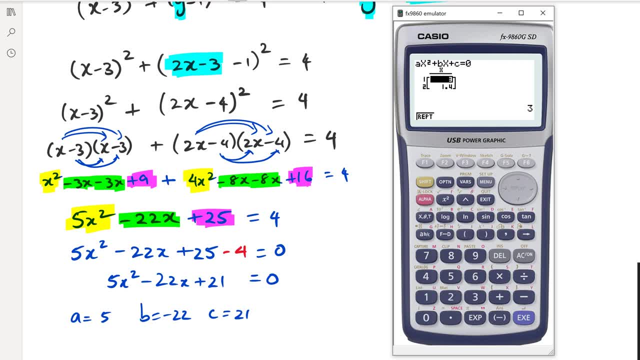 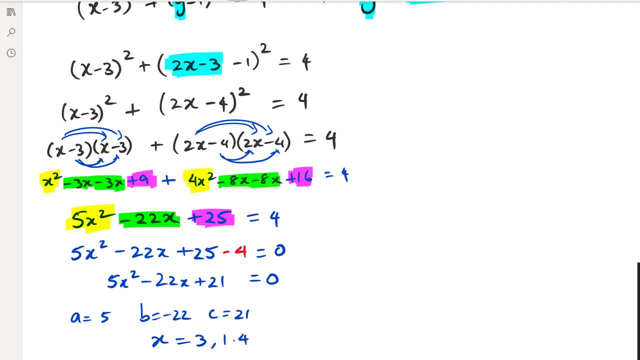 So there's my two answers where x equals to 3, and x equals to 1.4.. Now, remember, guys, we said we're going to use the straight line, right? So I'm actually going to put down: x is equal to 3,, x equals to 1.4.. 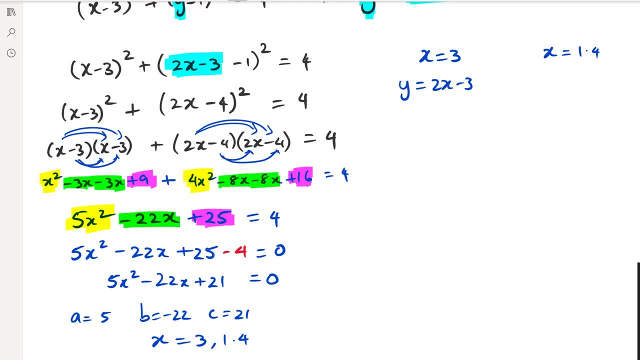 And then I'm going to write my equation down: y equals 2x minus 3.. y equals 2x minus 3.. So here I'm going to get: y is equal to 2 times 3 minus 3, which means I end up with a point of 3, 3.. 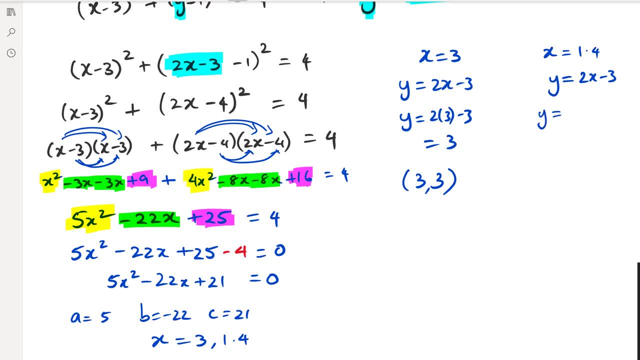 That's my first point. My second point is: y equals 2 times 1.4 minus 3.. That's 2.8 minus 3, which is negative 0.2.. So my second point is: y equals 2 times 1.4 minus 3,, which is negative 0.2.. 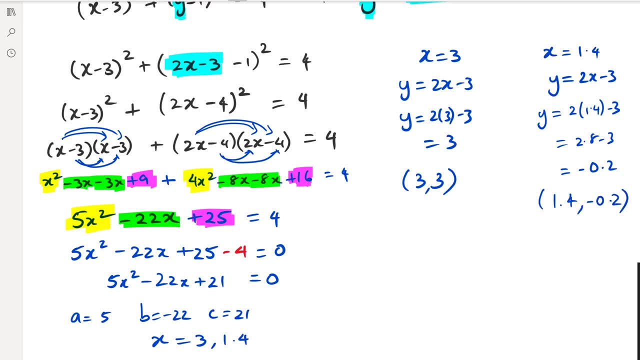 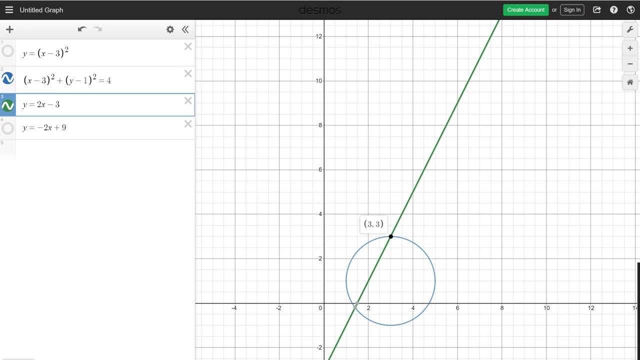 So my second point is 1.4 and negative 0.2.. So let's have a look, If I go back to my two things, So see how those two points actually pop up there. So it's 3, 3, and 1.4 and negative 0.2. 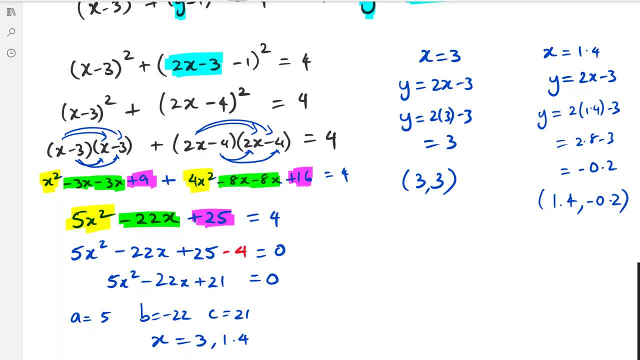 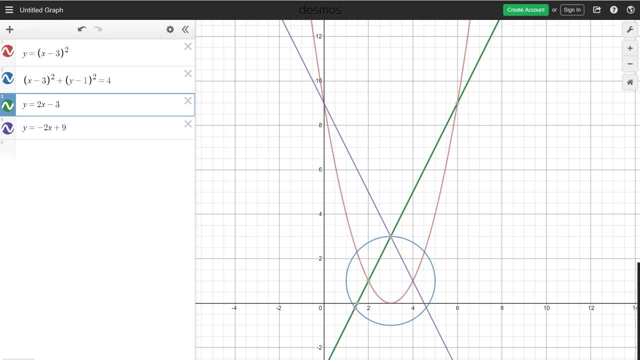 And those are the two points that I've actually got there. Okay, guys, I'm going to stop. I'm going to stop here for this particular video here, because what I would like you guys to try and attempt is now that I've shown you guys with the green line and the red green and the blue, 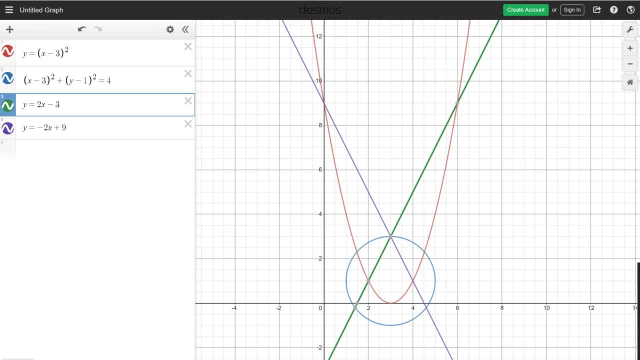 what I would like you guys to try is the purple line with the red parabola and the purple line with the blue circle, and have a go and see whether you actually get the right answers. okay, So just follow the same, working out as we did. Cool. That's it for this little video here. 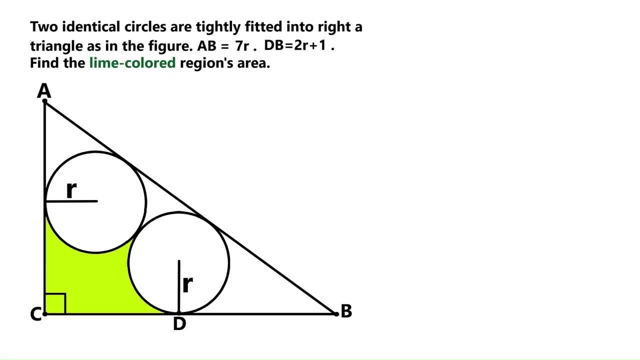 This geometric problem is absolutely fabulous, so make sure you don't miss any part of it. We've got this right triangle and these two identical circles are crammed inside the right triangle. Their radius is r and we are told this side ab is 7r and that this segment down here is 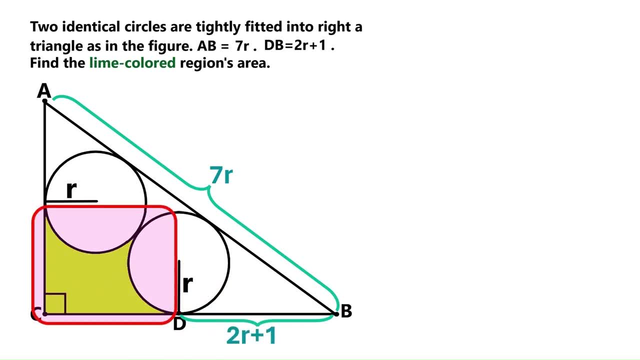 2r plus 1, and we've got to find the area of this weird shade lime colored region. So if you want to try this on your own, now is the time to pause the video, because I'm starting to solve it right now. This segment and this segment are both tangents to this circle and they both originate. 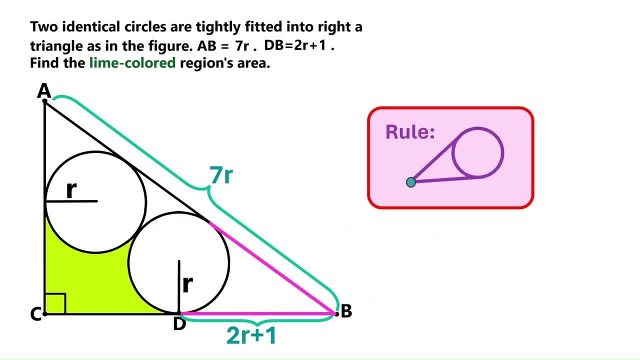 from this point b. We've got this rule in geometry that if two tangents are coming from the same point, their lengths must be equal. So we can conclude these two segments are equal and that this segment is also 2r plus 1.. We know this entire side is 7r, so this part over here has